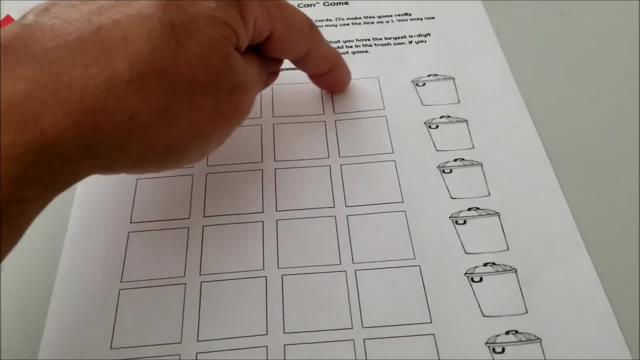 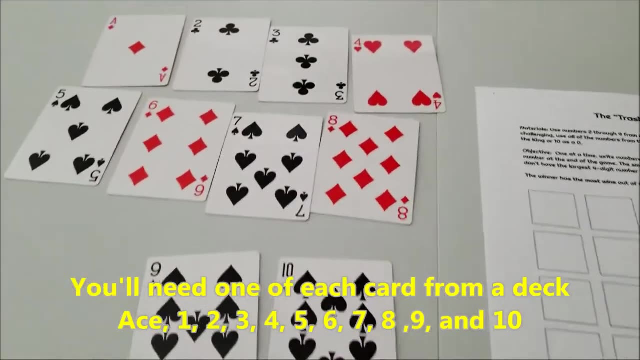 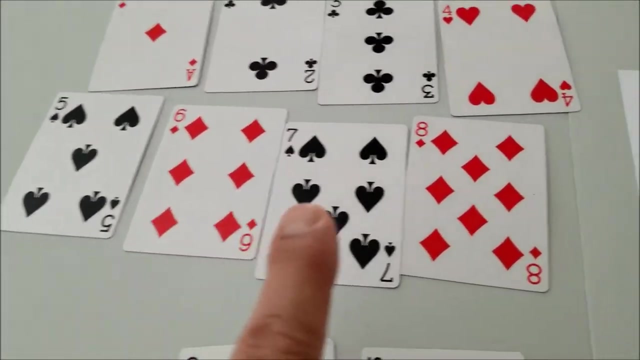 don't want to print it. you can just get a piece of paper and just draw four boxes and a trash can. No big deal. That's all I did, Okay, and then you're going to need also some playing cards You're going to try to get. we're going to use Ace as 1,, 2,, 3,, 4,, 5,, 6,. 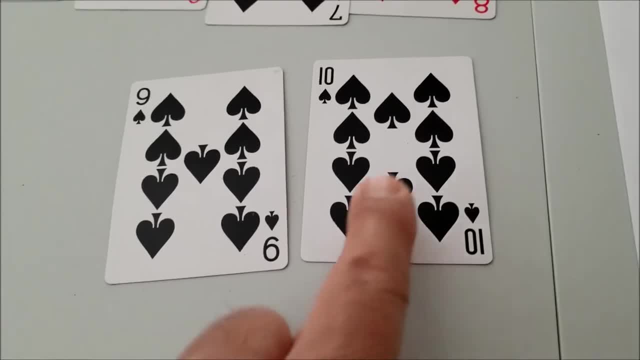 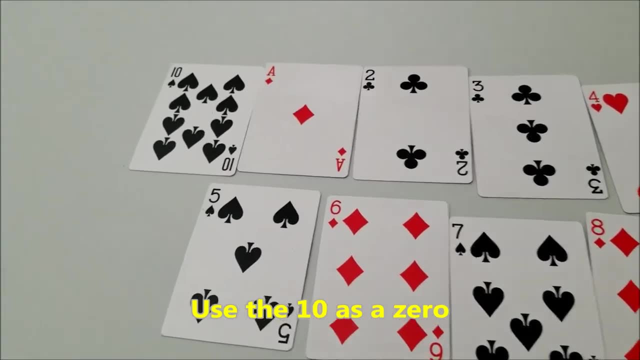 7,, 8., 9,, and then I use the 10 as a zero. So I'll actually put this up here. They don't have a zero in a deck, so I just use 10 because it has a zero in it. You can also use a king. 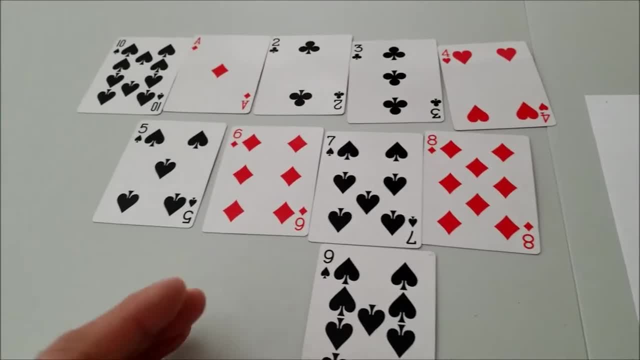 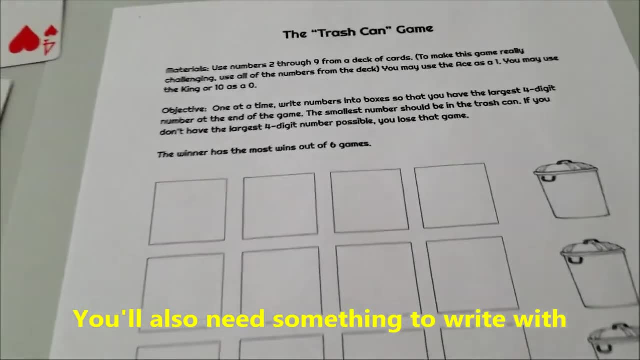 as a zero. It's up to you. But what you're going to want is you're going to want numbers zero through nine, and that's all you need. So let's go ahead and figure out how to play. So, basically, a game will consist of four boxes and a trash can. So what we're going to do, 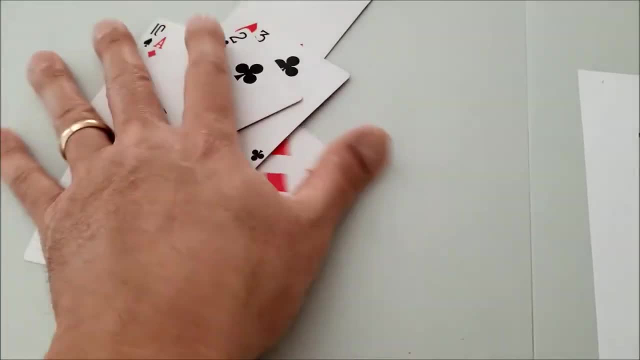 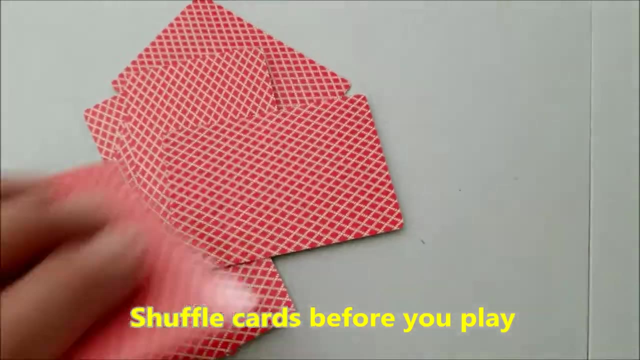 is, we're going to take all of these numbers and we're going to basically now flip them over so we can't see it. Nobody is supposed to know what any of these numbers are going to be. We're going to want to shuffle them, We're going to want to make it so that nobody 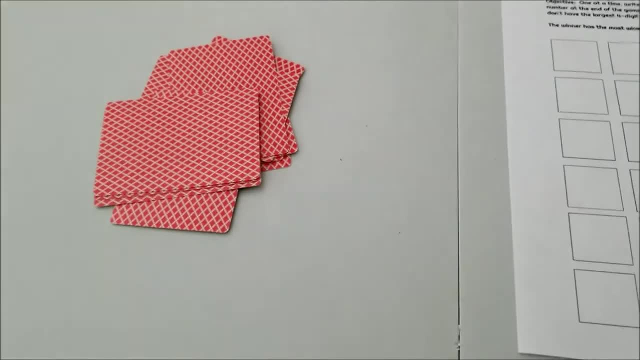 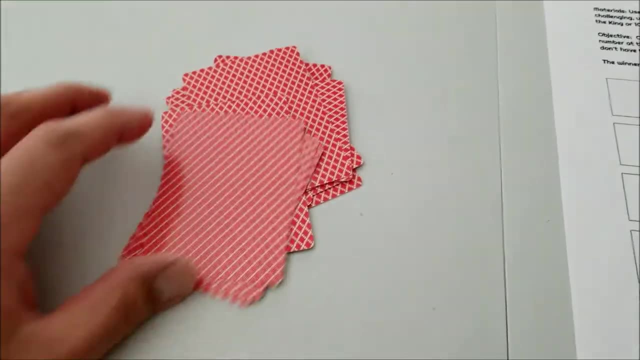 knows what card's going to get picked. So here's basically how you play. You're going to uncover your deck's going to look better than this- I'm trying to hold my phone here, so that's why I can't get a perfect deck- So you're going to flip the cards and you're 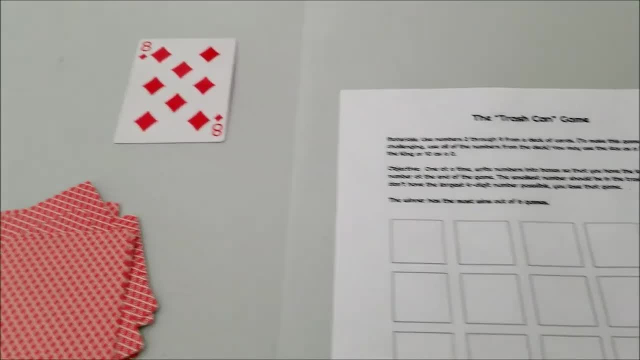 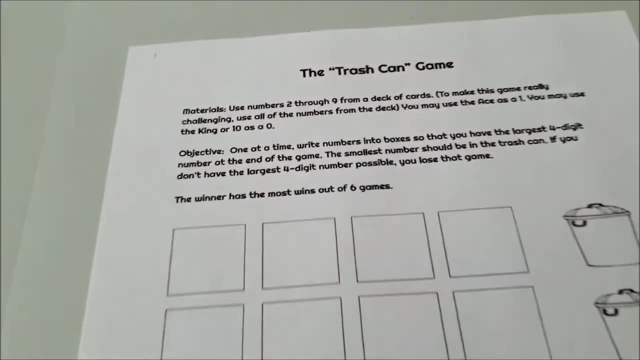 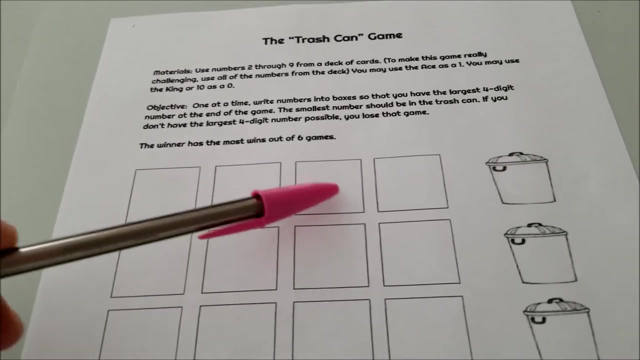 going to turn it over and, whatever that number is, you have to place that number inside of a box and your goal or your objective is: once we're done with the entire game, we're only going to flip over five cards- One, two, three, four- and then a number will get placed. 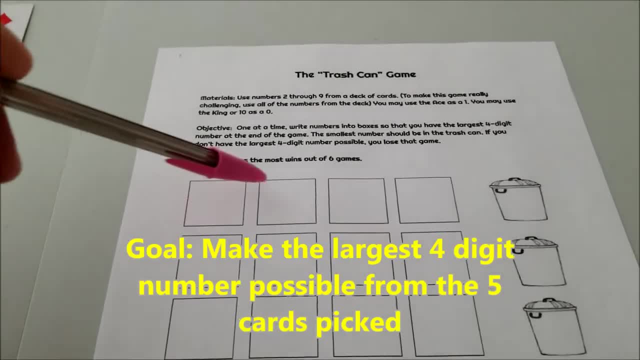 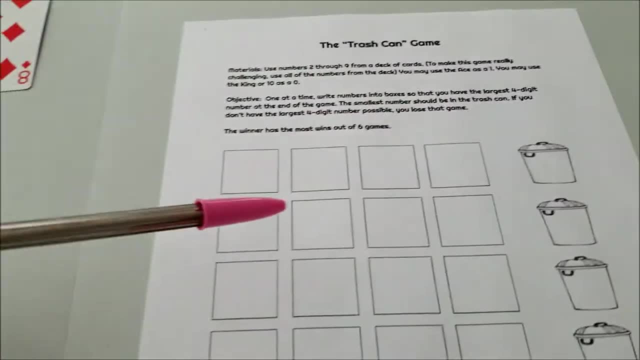 into the trash. Your goal is to have the largest four-digit number possible and the smallest number is going to be the largest number. So you're going to flip over five cards and you're going to be in the trash. So here is our first number. It's an eight. Now here. 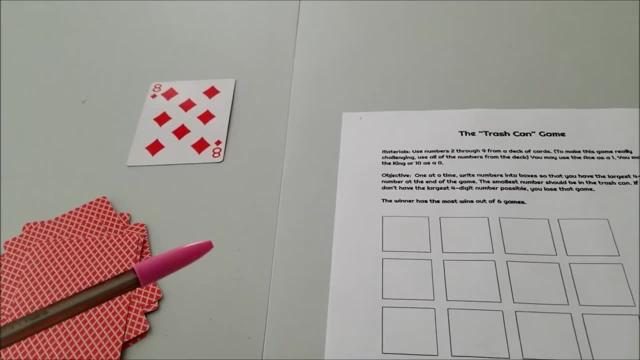 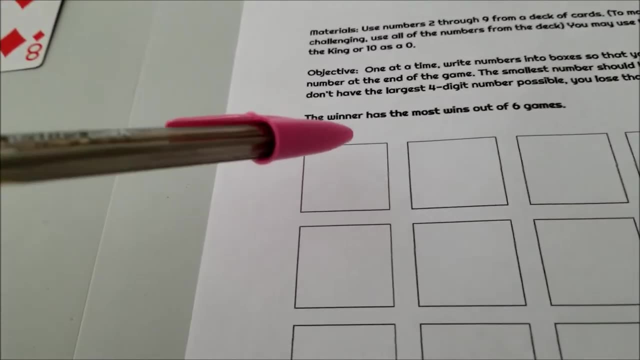 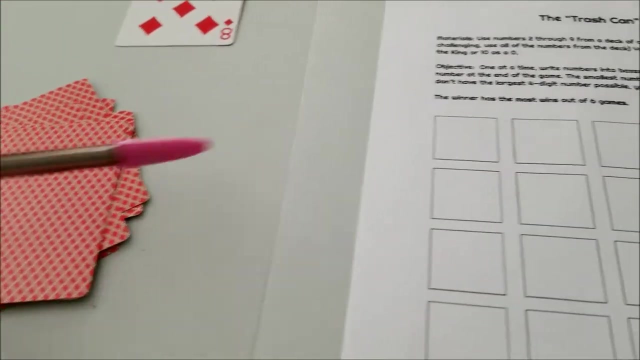 is where some thinking and definitely some luck is going to be involved. Now, the only number that's higher than an eight is the nine, And if a nine is picked, we'd want to put it here. If we put the eight here and we somehow pull over a nine, we won't have 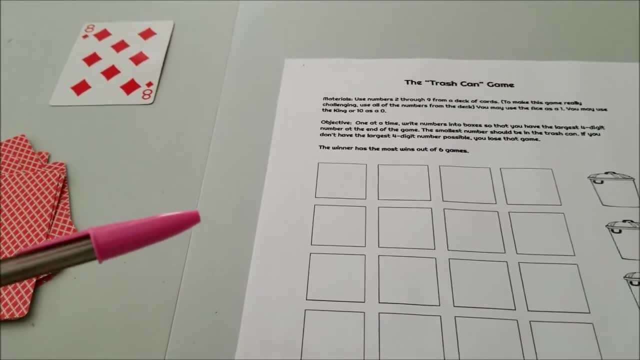 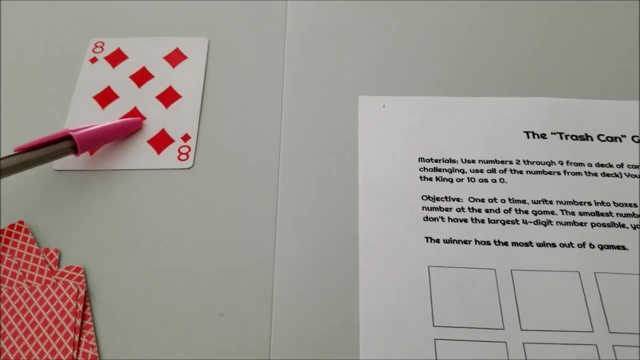 the largest number possible. So that is where strategy and strategy are going to play out, And definitely some luck, you know, is involved. So right now, that's what you would have to decide. If we pull over an eight, do we think the eight is going to be the largest number? 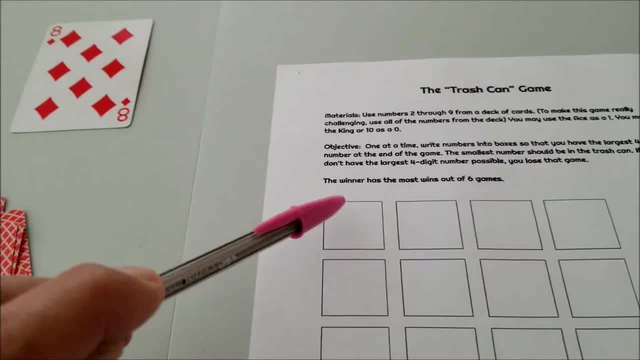 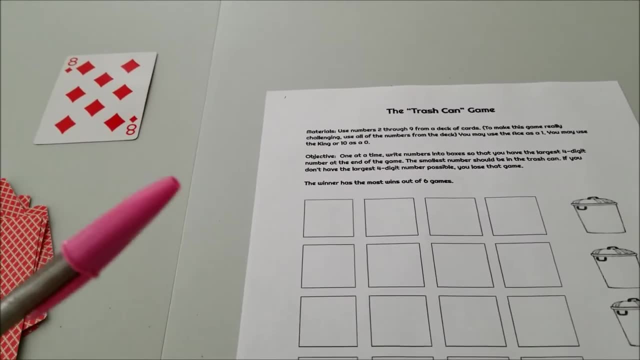 picked? Or should we put the eight here, assuming that maybe the nine is going to get picked? So we're going to get a chance to play this in a second, but let's just go ahead and flip the cards over. So let's just say, for right now, let's just go ahead and put an eight. 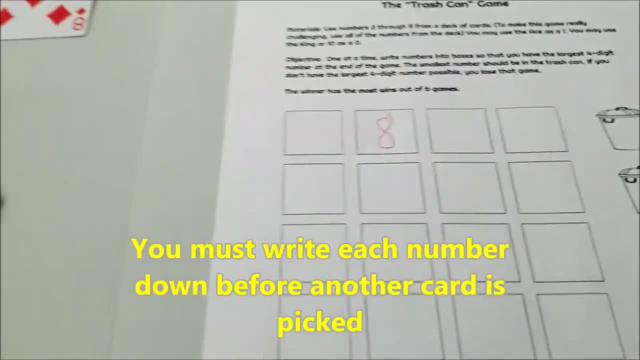 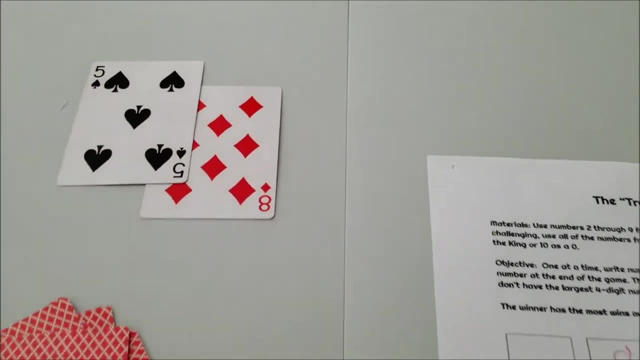 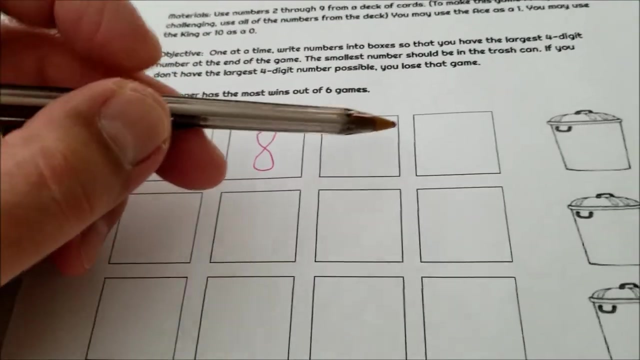 right here, And what we're going to do is we're going to make room for a nine if a nine does get picked. All right, let's flip over another card. Okay, so we got a five. The question is: okay, do we put the five here? Do we put the five here? Notice that we could actually 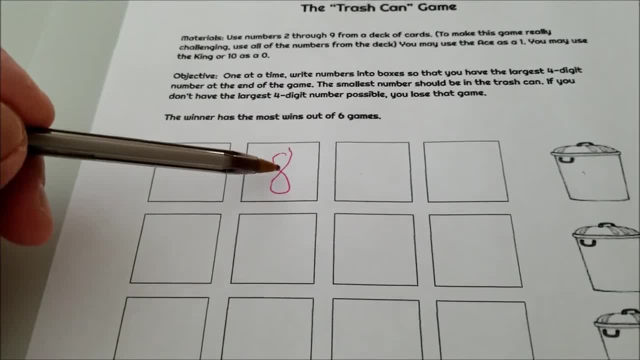 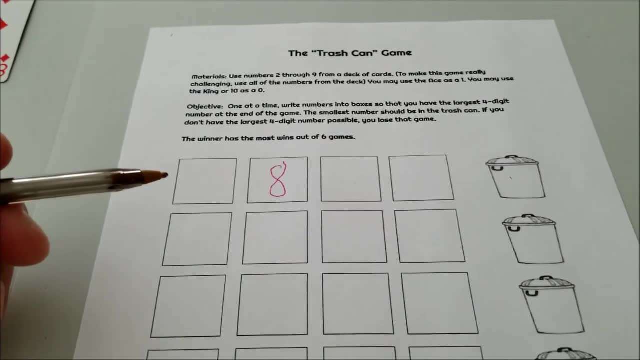 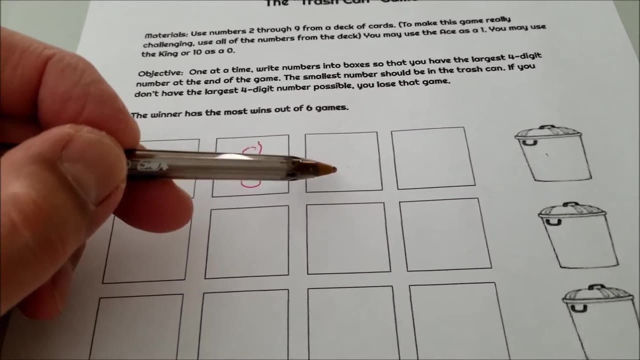 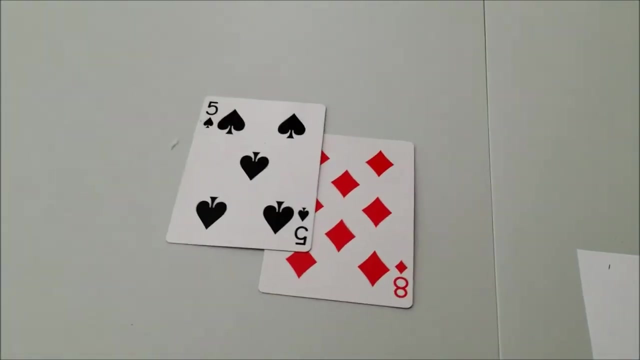 end up putting a five here, because numbers less than eight are seven, six, and then we could put the five there. I don't know what the odds are of getting that, So what I want to do is I want to make room for a seven or a six, So I'm going to put the five right there. Okay, now we're. 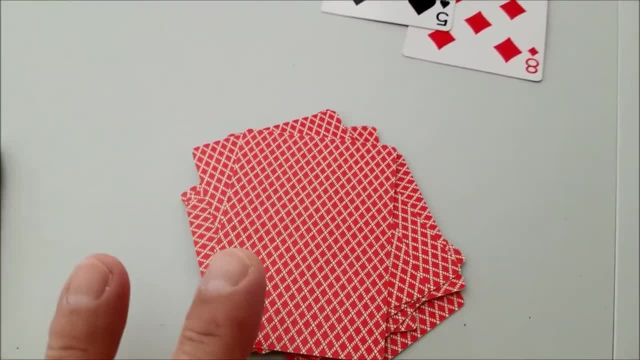 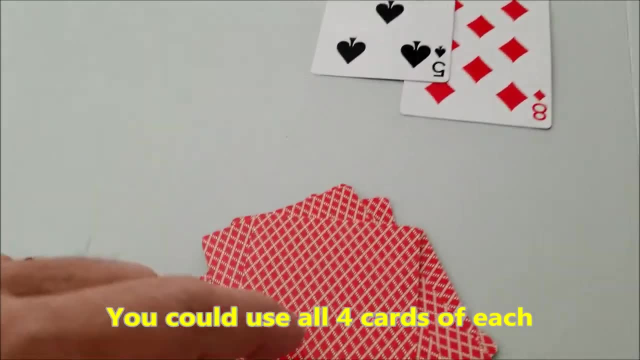 not going to mess with. if you wanted to make this game more challenging, what you could do is use more decks of cards and get out. I'm sorry, use all of the numbers from the entire deck. Notice, I only put the five here. 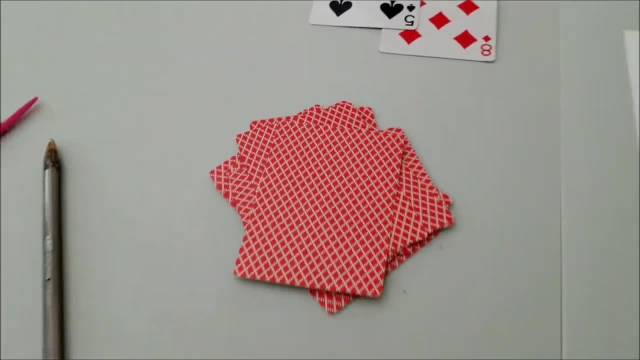 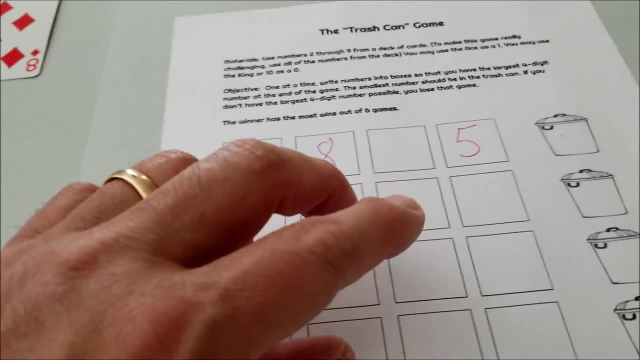 I pulled out one of each card. If you wanted to make this more challenging, what you could do is pull out all of the fives, all of the eights out of a deck. That way there's a chance of pulling another five, But for right now we've only got one of each. Okay, so, 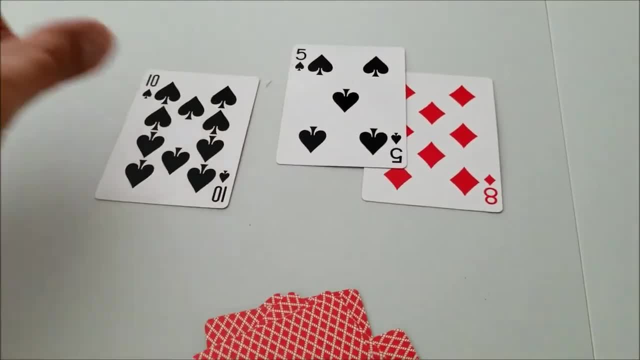 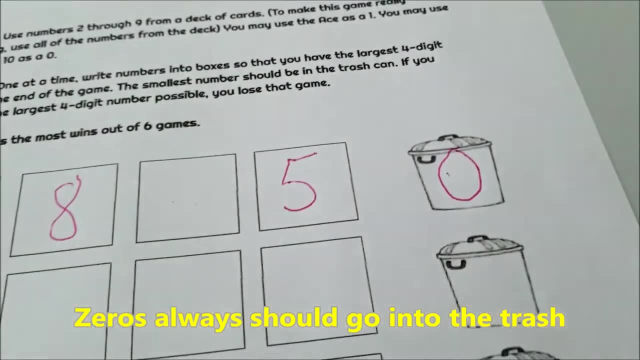 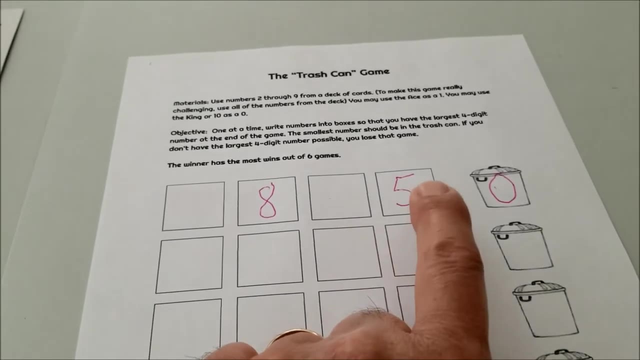 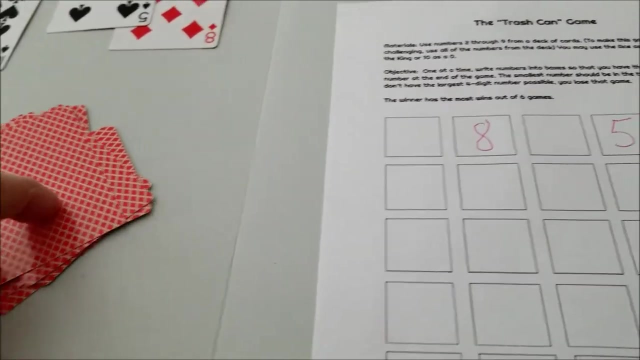 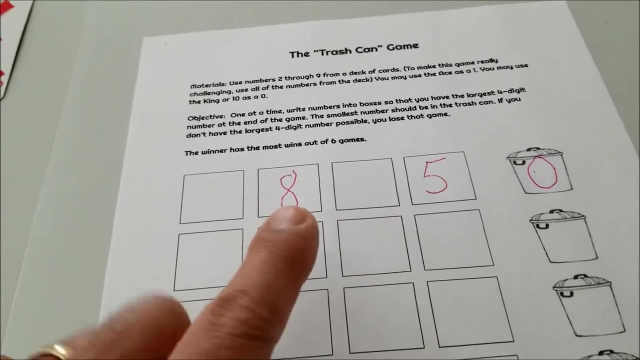 here's the next card. Okay, so remember, that's a zero, And what's good about that is there's nothing smaller than a zero. So we're okay putting that in there. We're okay putting that in the trash. Now, with the way we have this set up right now, the only bad thing is if a four, three, two or a one is picked out of this deck, we've automatically lost because I put the five there. So I'll show you when we're all done how I know who won, or if we won. Okay, let's pull the next card. 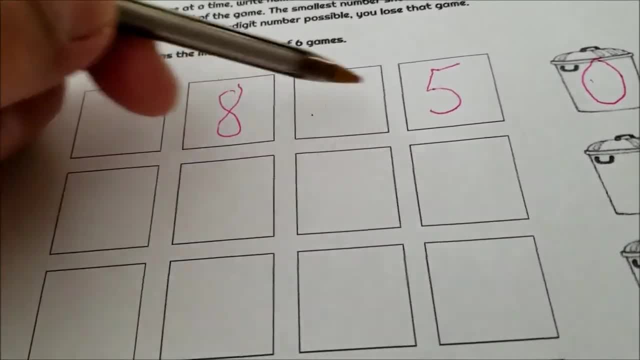 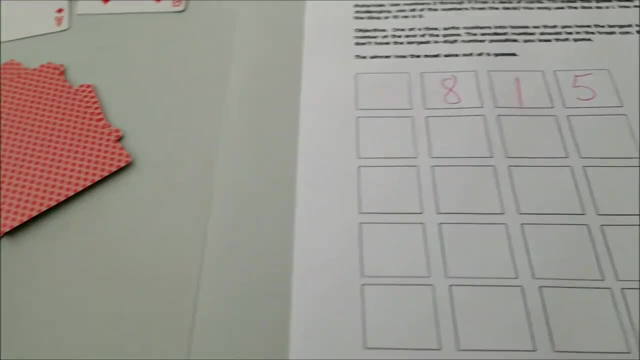 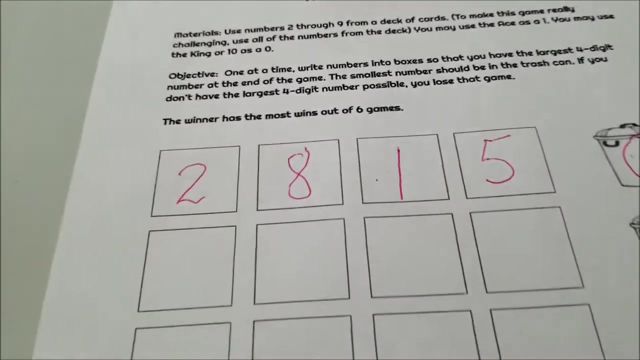 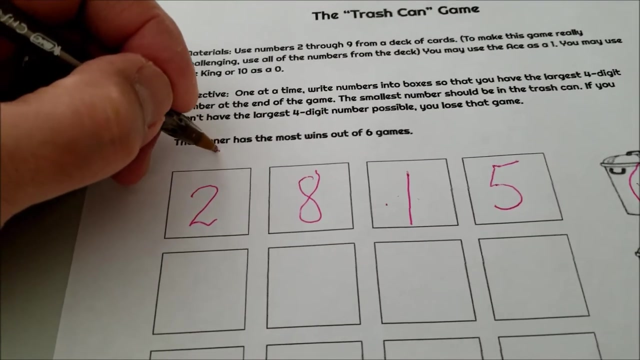 There was a one. I should have put the five here, so I had a place to put the one. So everybody guess what This game is automatically done. I'll just pull this last one, just to be sure. Okay, so the numbers that were picked were two, eight, one, five, zero. The largest number we could have made would have been an eight, a five, a two. 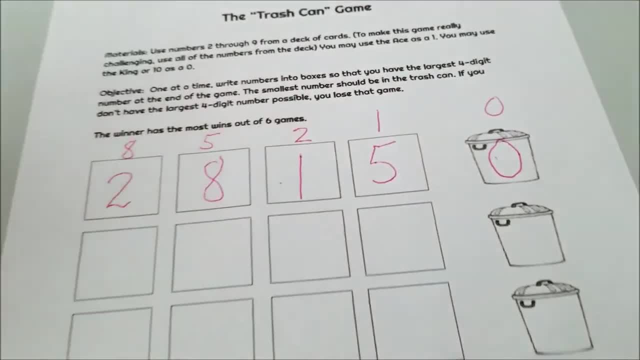 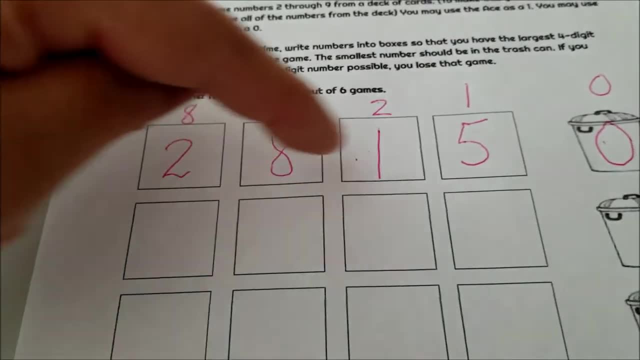 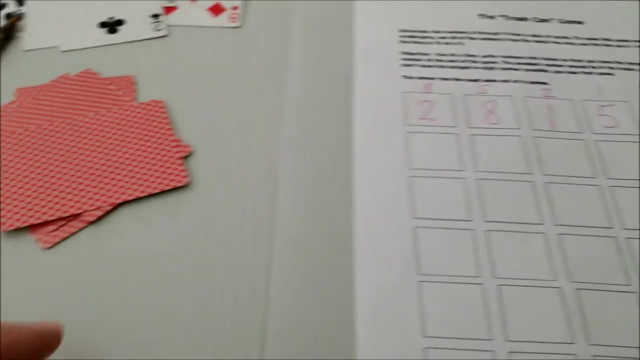 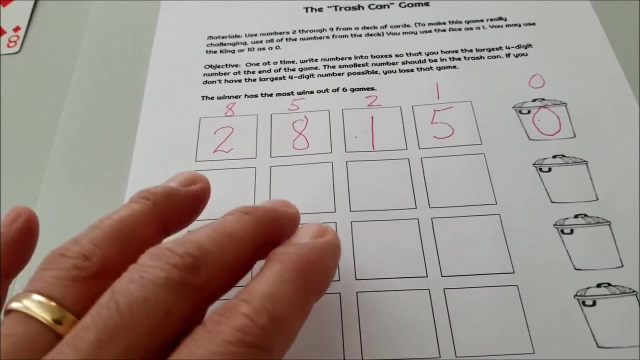 a two, a one, and the zero we did put in the right place, So that would have been the winning number right here: Eight five two one. We didn't have that set up so we lost. So you can see how this game is super challenging. You never know what card's going to be under here and you have to kind of get lucky and definitely do some strategizing to see where should you put certain numbers. 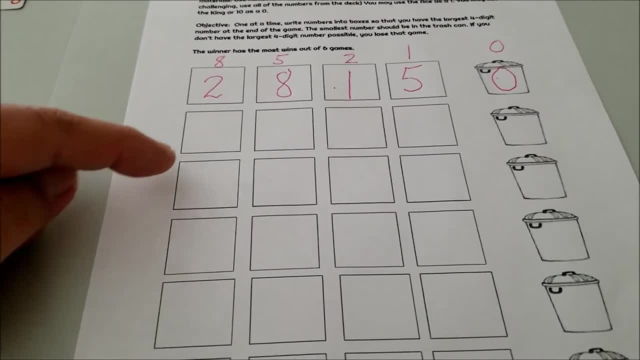 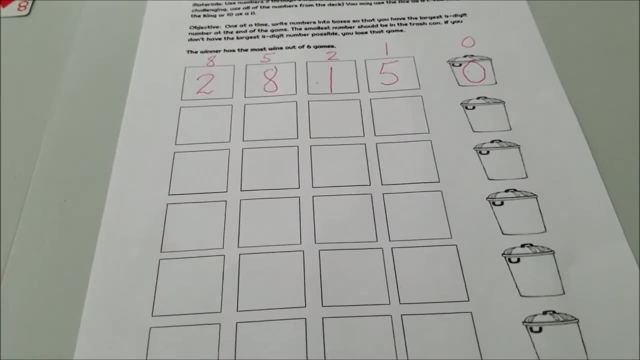 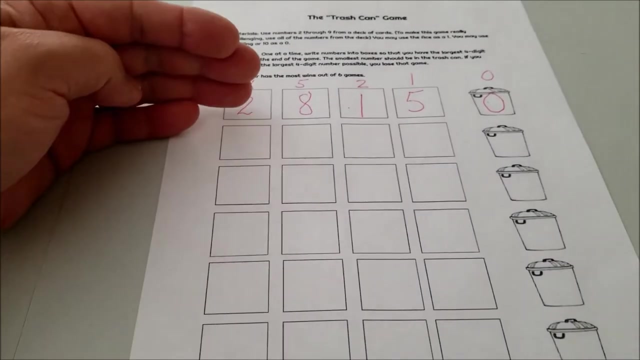 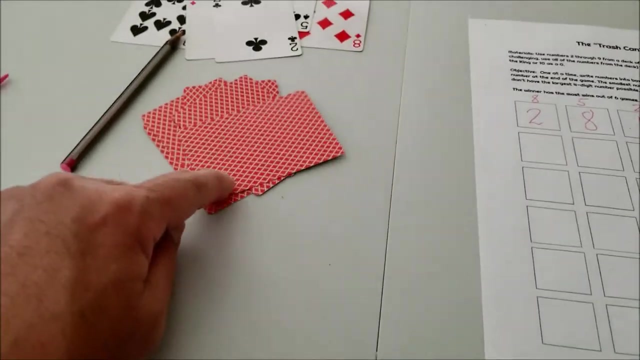 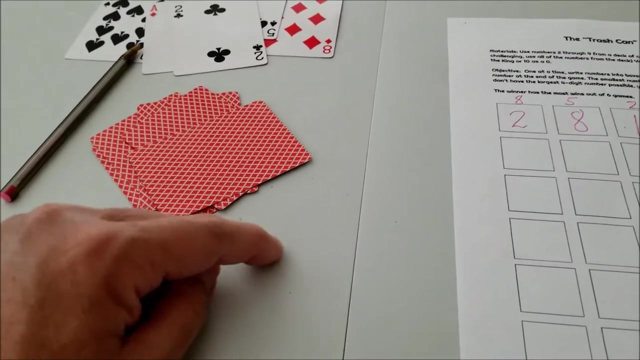 Okay, so that's the. that's basically the game On the paper. I've given you two, three, four, five. I've given you six basic games that you can play. Like I said, if you don't, you know you can always flip it over. You don't have to print this out again, but I have left you that link in case you want to keep printing these off. Teachers, you could print this off and photocopy it for students if you want, if they're allowed to have playing cards or if you don't have playing cards, you know you guys can just take a piece of paper and cut up. you know, just going to have to. 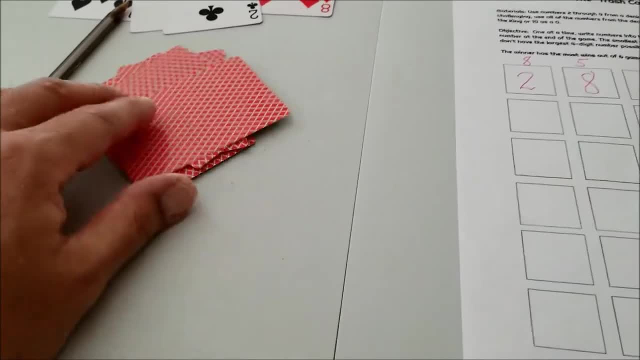 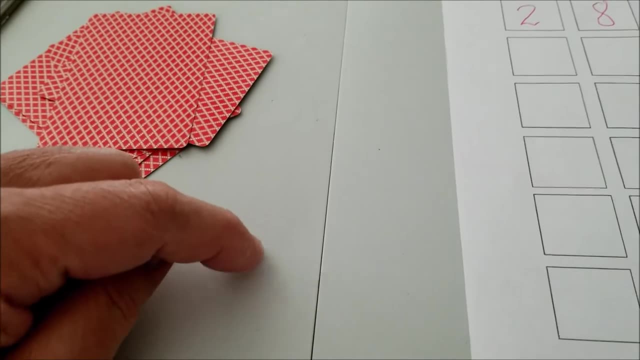 make sure you can't see the numbers you know on the other side of paper. The good thing about cards is you can't really tell which card this is. Pieces of paper you might be able to see that number you know. 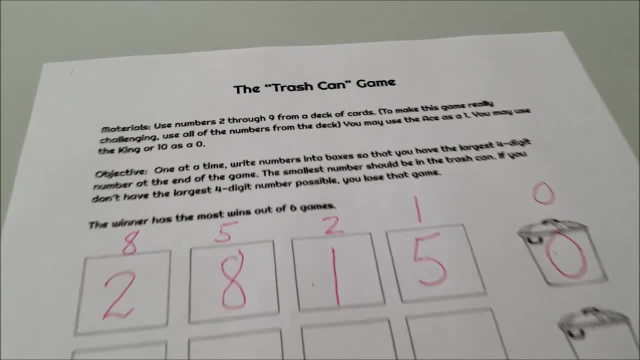 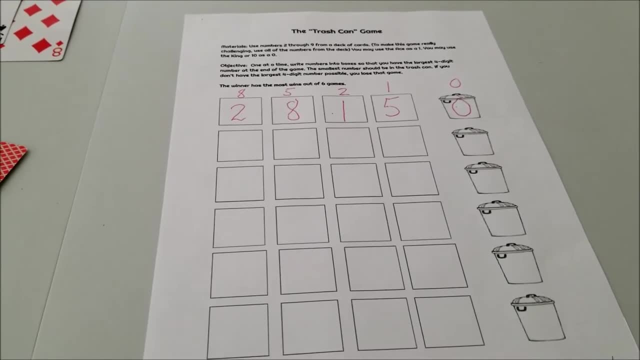 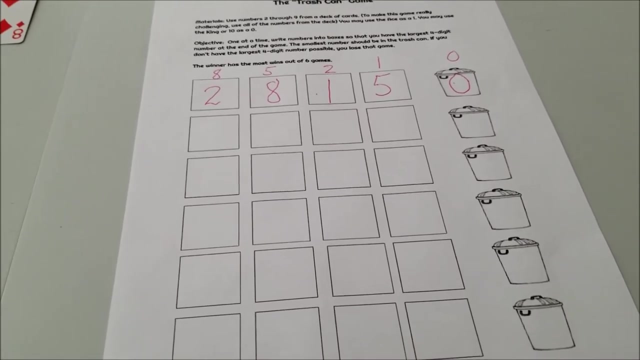 underneath it. so Okay, everybody. so that is the Trash Can Game. Definitely very challenging to win. It's just one of those things, though, but it's fun. I've taught math for 18 years- My students always, even though. 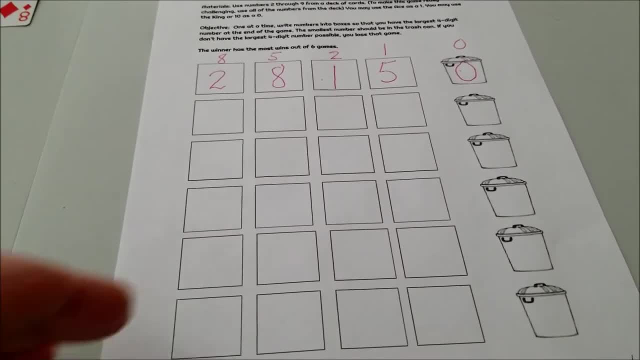 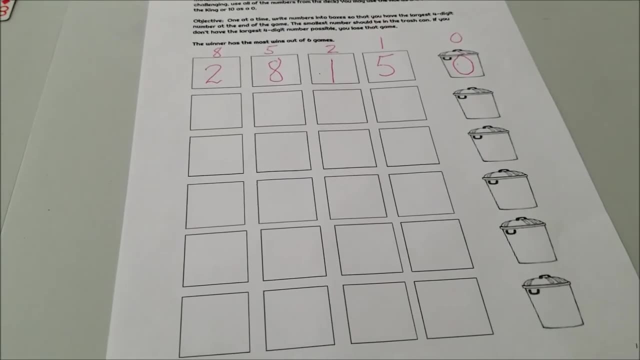 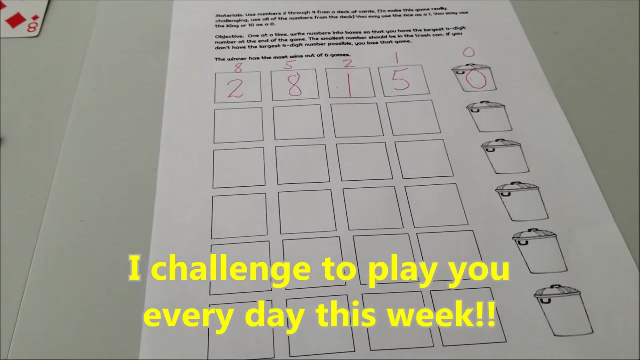 was frustrating at times. they always seem to get excited to see you know how many games could they win out of these six games. to be honest, they were excited they could win two. it was really challenging. so what i also plan to do this week is to challenge you guys. i'm going to make a special. 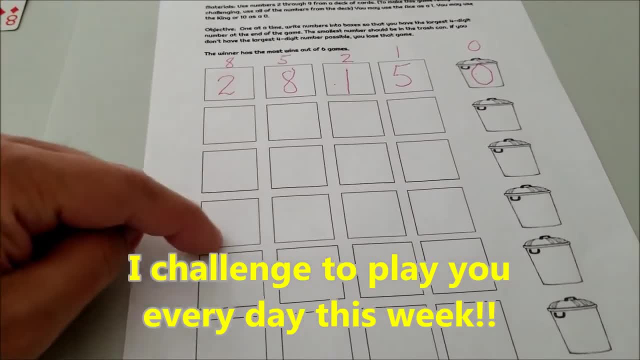 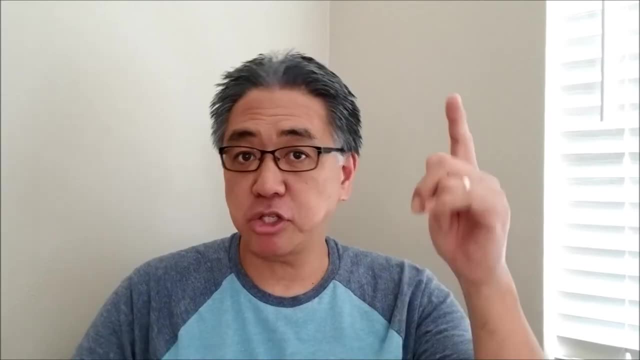 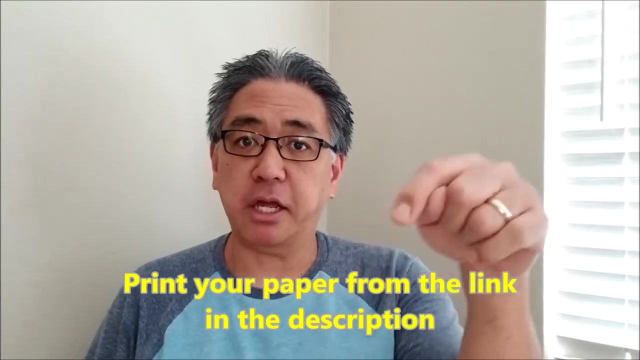 video every day where you get to challenge me on winning the trash can game. so stay tuned for the next video. okay, guys. so there's the trash can game- super fun. please, if you get a chance, check the description for the link. i'm printing this out, um, i'm just giving it away to you guys, just. 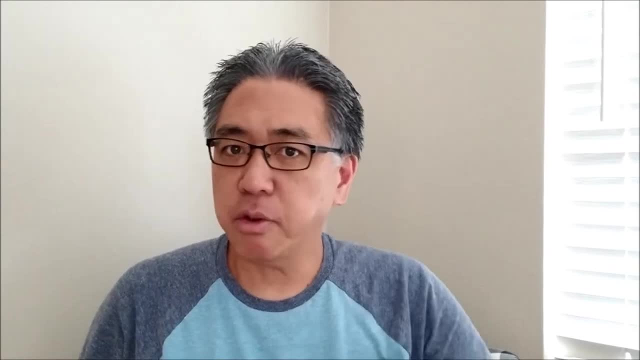 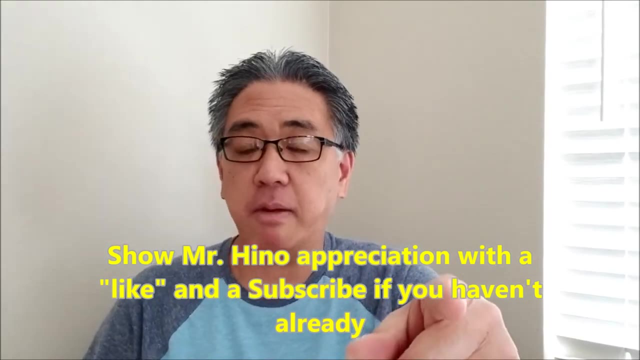 because i think it's fun and it's a just another way of saying hey, thanks for watching and if you're really appreciative, hit me up with a like too. okay, and definitely subscribe. okay guys, i am mr hino from mr hino's math. i'm gonna be with you. 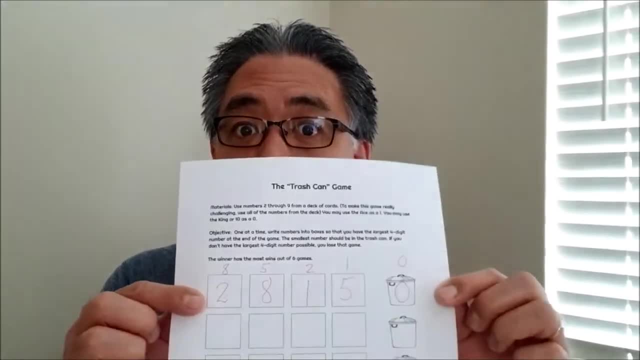 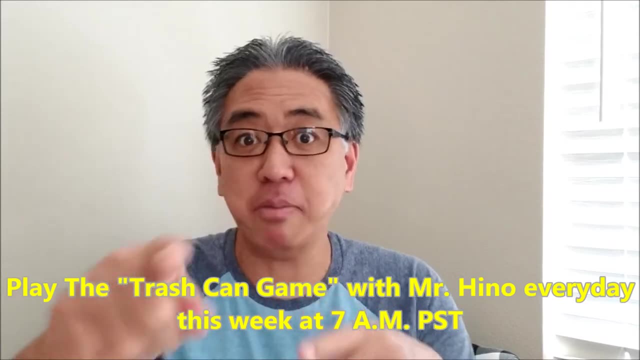 again tomorrow to play a game with you guys, where i'm we're actually going to make this for real- where you get a chance to play at home with me and i'm gonna see if i can beat you. yes, i'm gonna trash talk right now, just so that you'll tune in and try to play with me. okay, so i will see you. 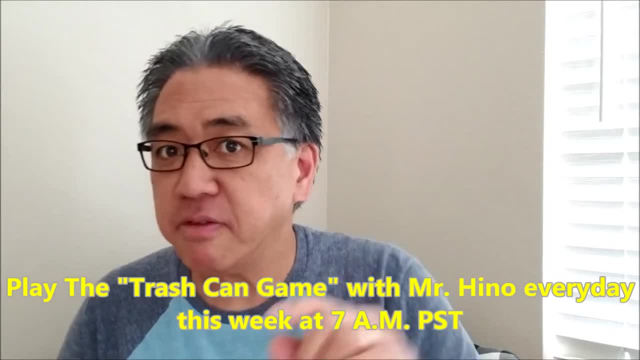 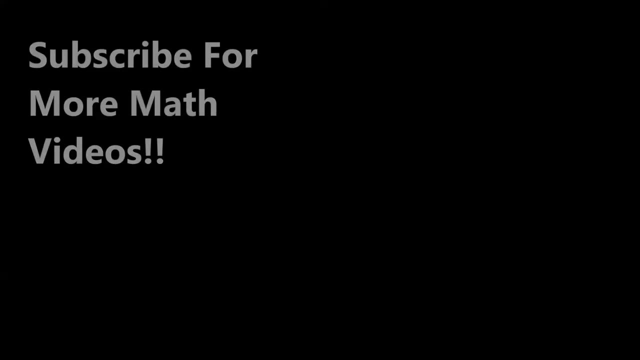 right here again. tomorrow, seven o'clock pacific standard time, i challenge you to a game. okay guys? all right, i'm mr hino math. i'll see you tomorrow you.